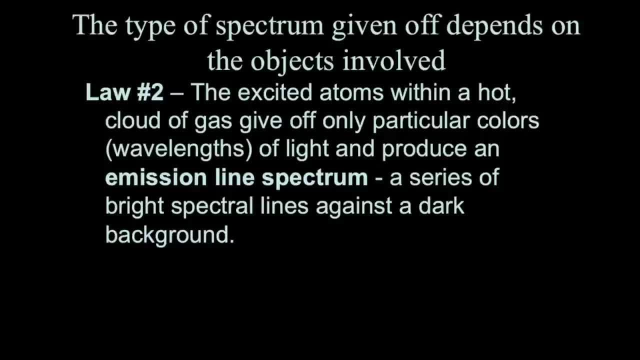 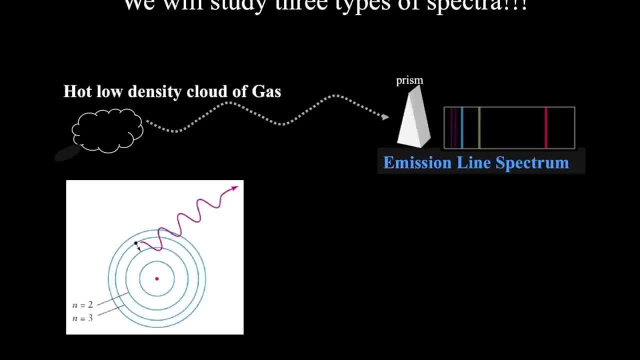 of certain colors, certain lines, and we have a black background. It looks like this: And so we have a hot, low density cloud of gas. For example, that could be a nebula in space. Well, that's only going to produce the specific colors that the atoms in that. 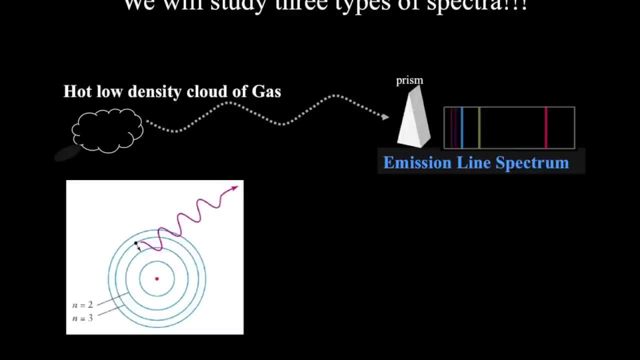 cloud are sensitive to. So we have a hot, low density cloud of gas, For example, that could be a nebula in space. Well, that's only going to produce the specific colors that the atoms in that cloud are sensitive to. What's happening at the atomic scale is that electrons in those atoms in the cloud of 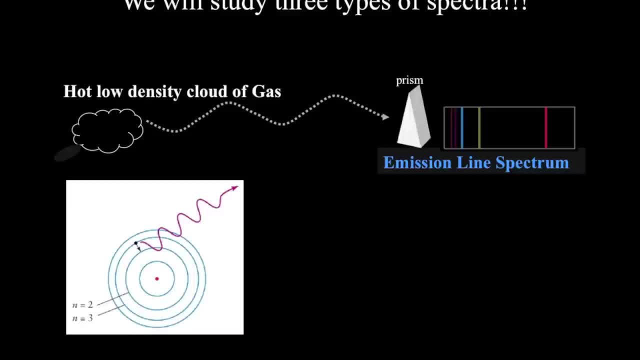 gas have been energized, and then they're dropping down levels and emitting photons of light. Individual atoms may be able to emit more than one color of light, but they're not going to produce an entire continuous spectrum, And so what we'll see is an emission. 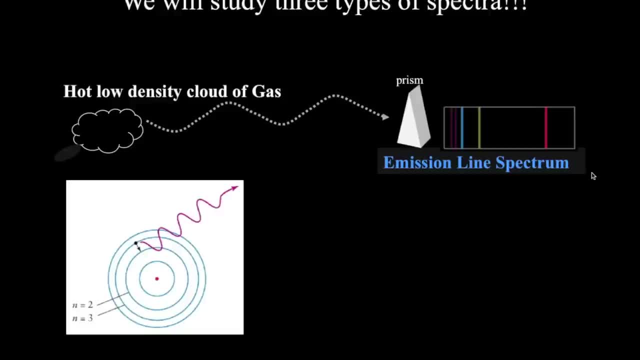 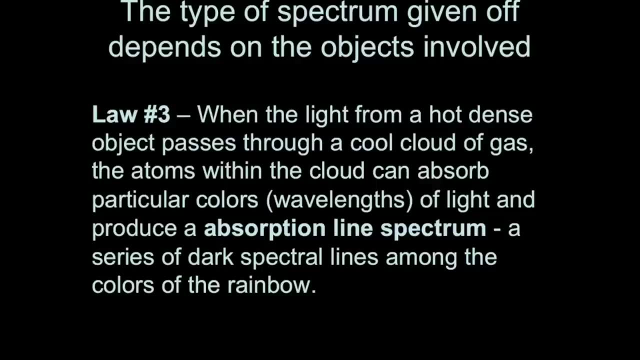 line spectrum, like we have here on the right, It looks like bright colored lines on a dark, dark background. Finally, if we take the light that's produced from a continuous source and then pass it through a lower density and cooler temperature cloud of material or cloud, 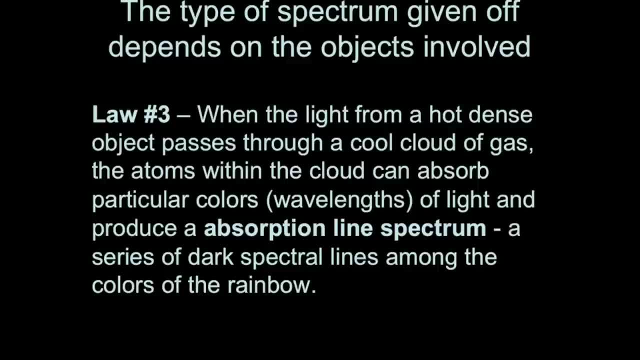 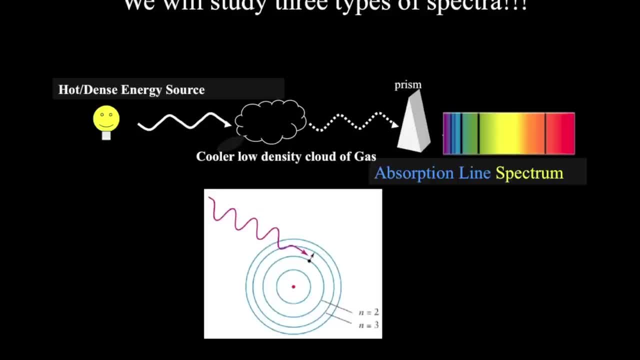 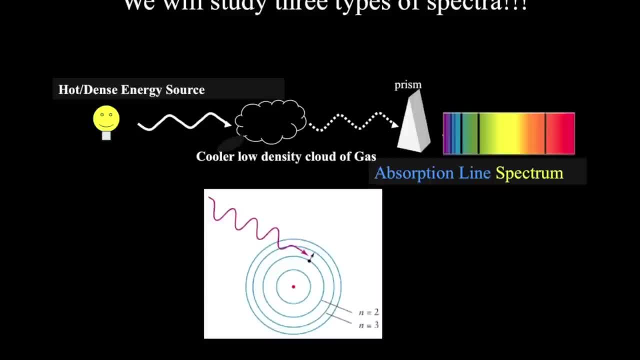 It looks like this. Let's say that we start with the continuous light coming from a hot, dense source. We pass it through a lower density and cooler collection of atoms. Those atoms will absorb the colors that they are sensitive to. It's not going to be every color, just some of. 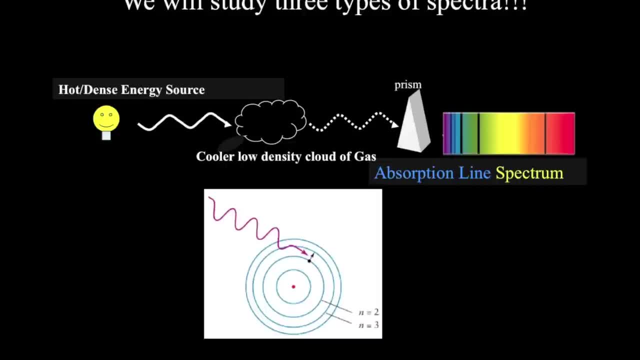 them. And so, on the other side, if we take the emerging light and pass it through a prism or a spectrograph, what we'll see is what appears to be a continuous background with certain colors. And so, on the other side, if we pass it through a prism or a spectrograph, 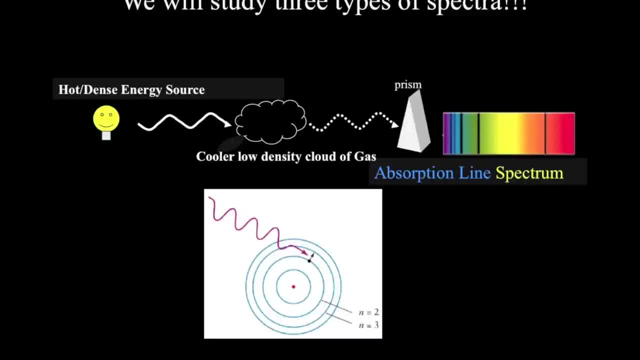 we'll see that all of these colors are removed. an absorption line spectrum At the atomic level. what's happening is that when all of that light- essentially white light- passes through the cloud of gas, the atoms in that cloud of gas absorb certain